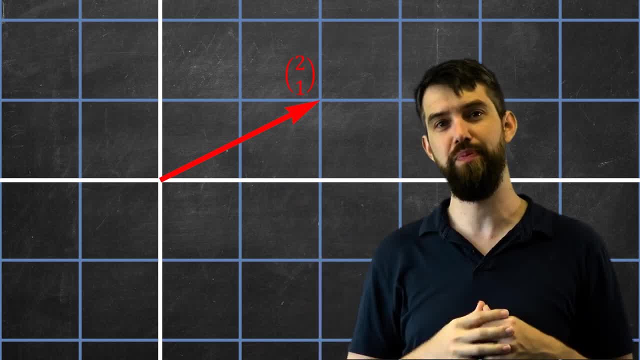 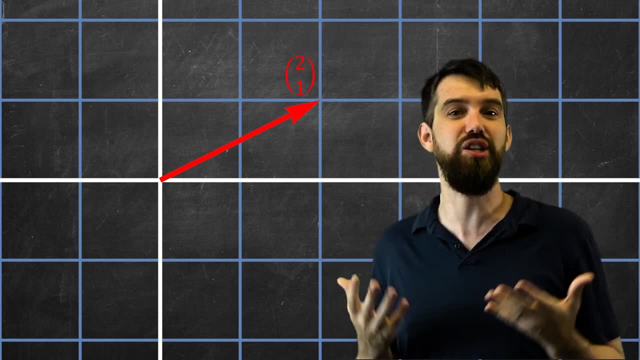 starts at the origin and then goes up to this point: 2, 1.. And now, instead of writing it horizontally, I typically write this vertically. this 2, 1. And 2, 1 is the x and y values of the end point of this little arrow that I've drawn. 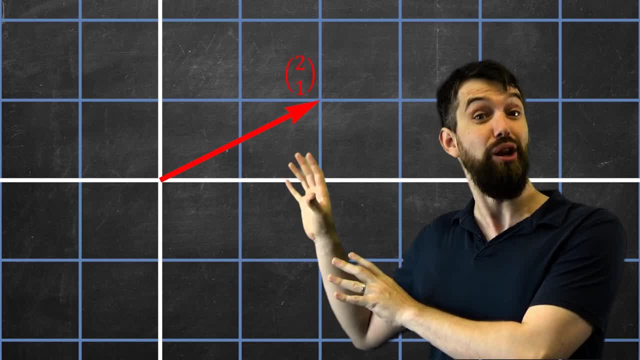 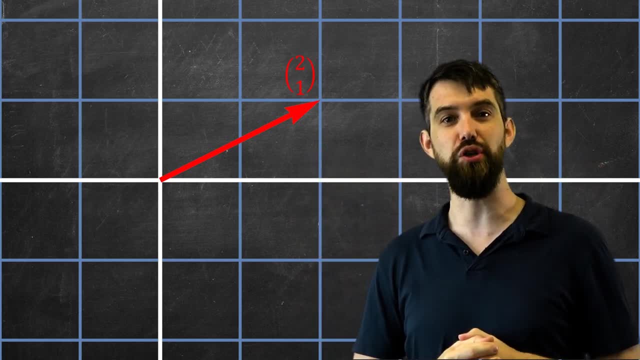 But the key thing is this: This vector, this little arrow that I've drawn here, I don't only want to think of it as starting at the origin and going out to this particular point 2, 1.. So, for example, this vector here where I move it up, or this vector where I move it. 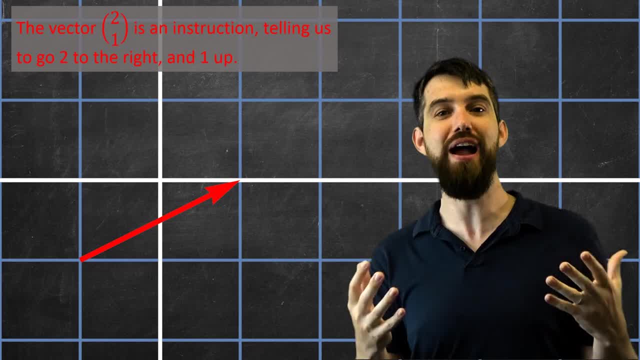 down. I want to think of these vectors as the same vector. They are an instruction. an instruction that tells you, no matter where you stay in the coordinate system, you'll always be able to do the same thing. I don't want to think about this vector as the same vector. They are an instruction, an. 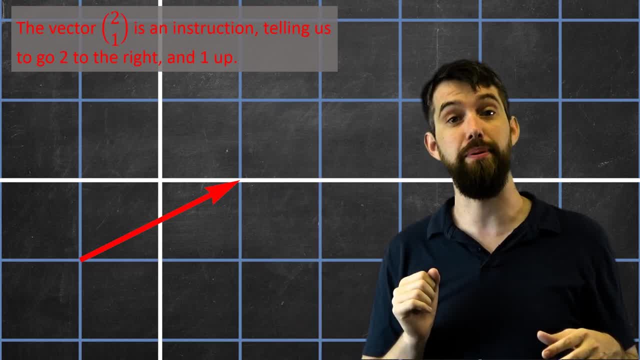 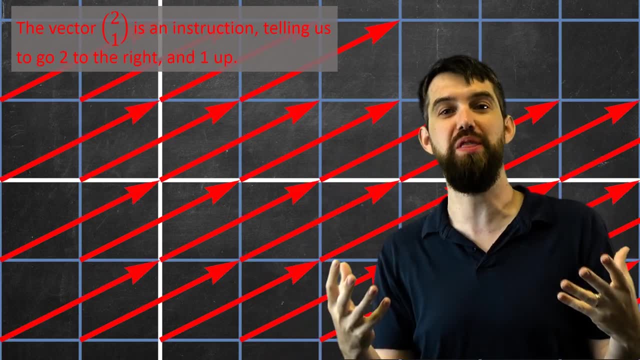 instruction that tells you, no matter where you stand, no matter where you move, you'll always start to go two steps to the right and one step up. Indeed, I can imagine that this vector could start anywhere on the plane and at every particular point on the plane, I'm going to have the instruction. 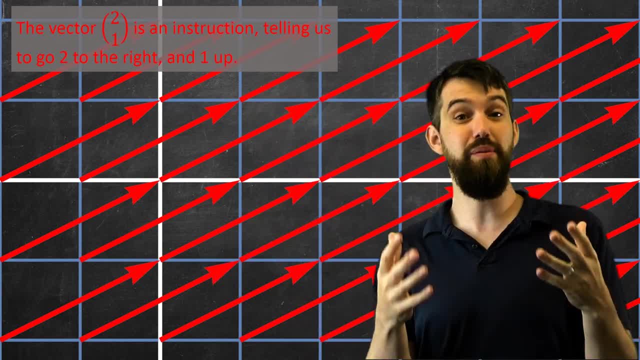 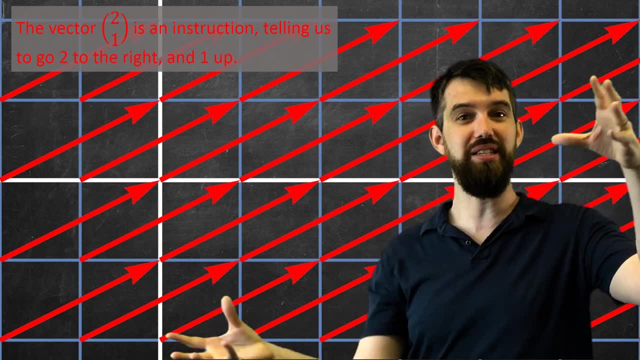 go the two steps to the right and the one step up. This may seem a bit strange, but think about gravity, for instance. Every one of us feels the effect of gravity and even if we're on opposite sides of the earth, there's some arrow, usually pointing approximately the center of the earth. 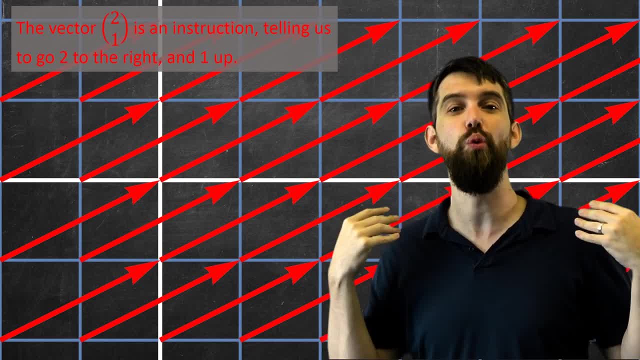 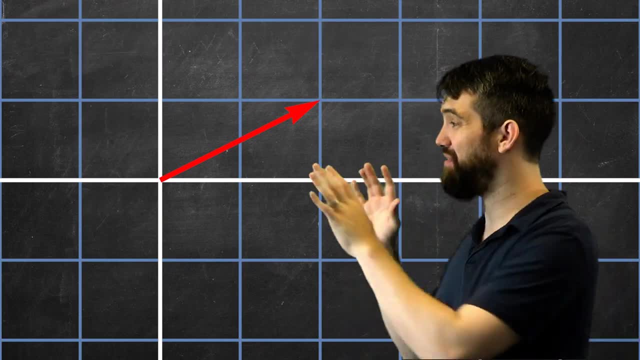 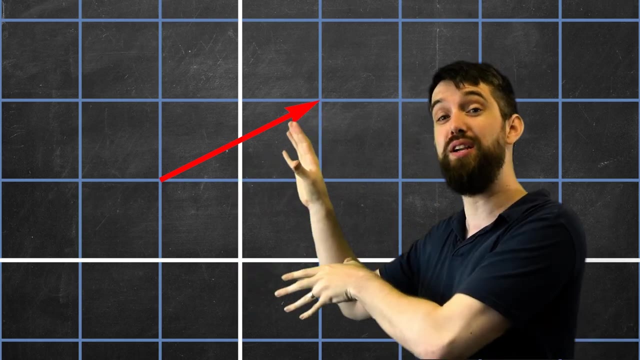 that tells us where we're supposed to go. It tells us which direction gravity has had an effect. Or, if I want to change my perspective a little bit further, I can think of this vector as the thing that's fixed and what's changing is the underlying coordinate system. The vector doesn't move, but the coordinate system. 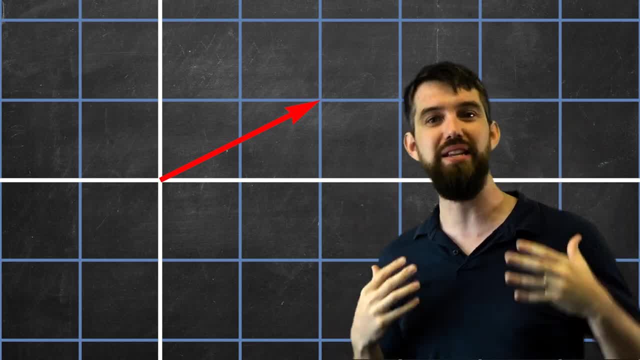 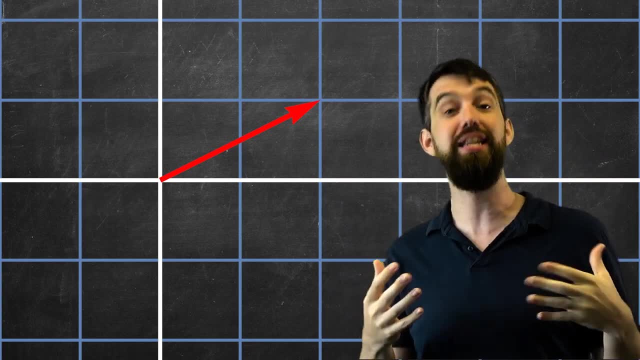 that's what moves, Sort of a way of thinking that you and I may disagree on what the origin is. I may put the origin where I am and you may put the origin where you are, but either way there's the same claim to take two steps to the right. 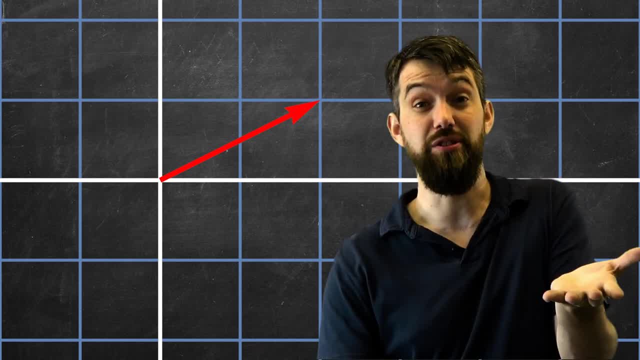 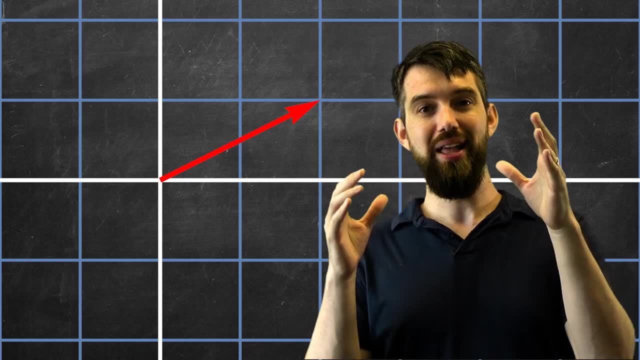 And one step up. All right, so I have these vectors, but what can I actually do with them? Well, one thing that I can do with them is I can stretch them. So, for example, if I take that same vector, the, and I stretch it out by a multiple of 2,. 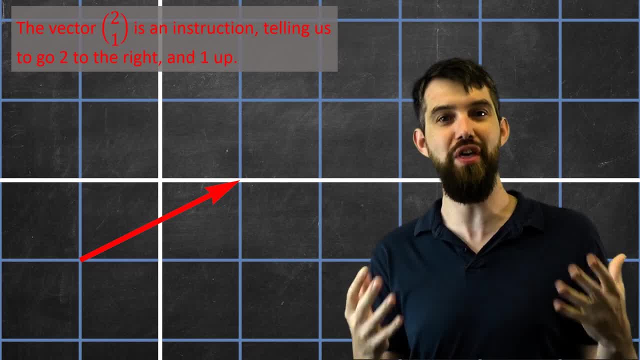 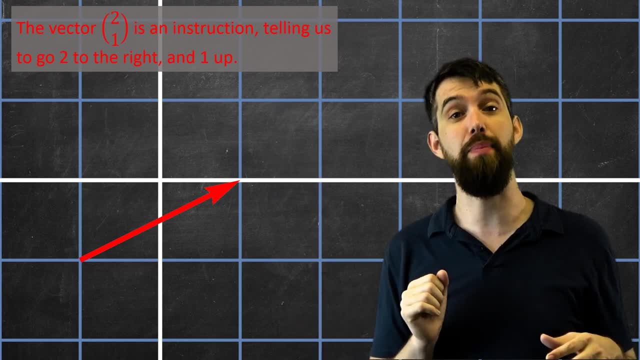 I want to think of these vectors as the same vector. They are an instruction, an instruction that tells you no matter where you start to go: two steps to the right and one step up. Indeed, I can imagine that this vector could start anywhere on the plane. 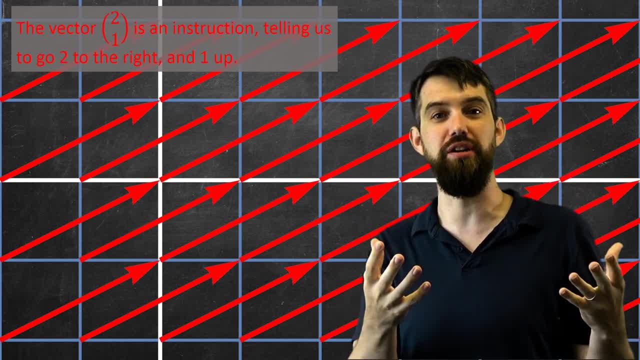 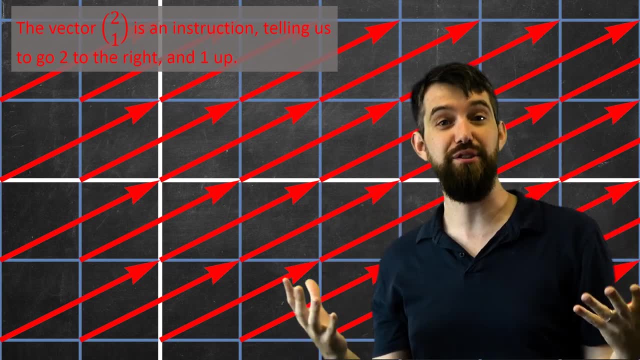 and at every particular point on the plane I'm going to have the instruction: go the two steps to the right and the one step up. This may seem a bit strange, but think about gravity, for instance. Every one of us feels the effect of gravity. 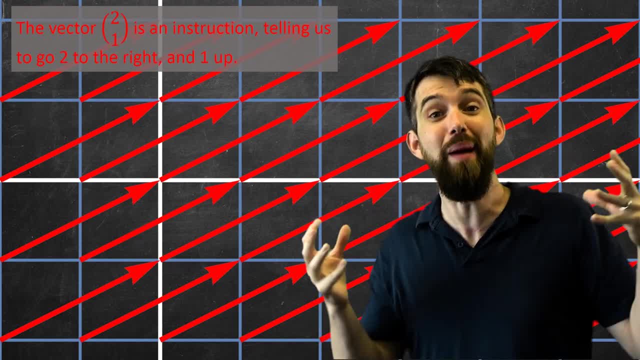 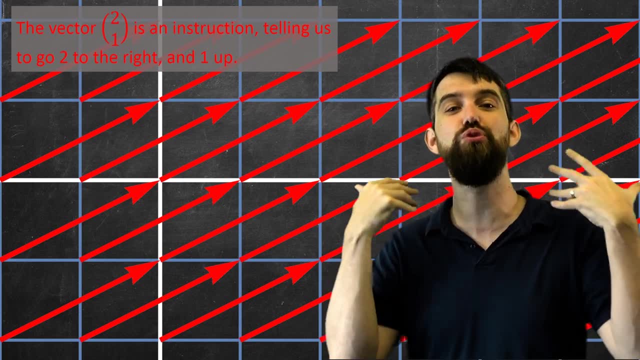 And even if we're on opposite sides of the Earth, there's some arrow- usually planets- pointing to approximately the center of the Earth. that tells us where we're supposed to go. It tells us which direction gravity has had an effect. Or, if I want to change my perspective a little bit further, 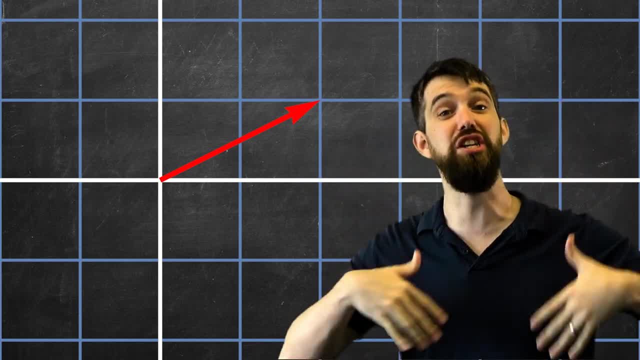 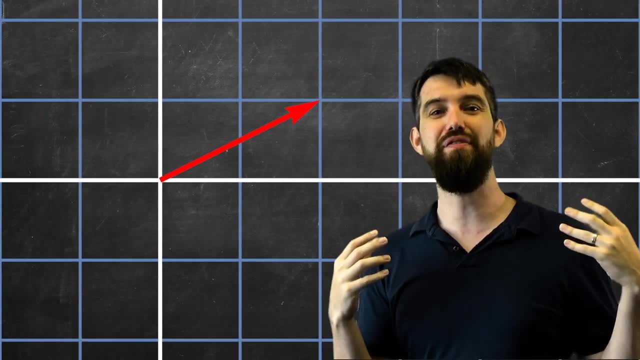 I can think of this vector as the thing that's fixed And what's changing is the underlying coordinate system. The vector doesn't move, but the coordinate system, that's what moves. It's sort of a way of thinking that you and I may disagree on what the origin is. 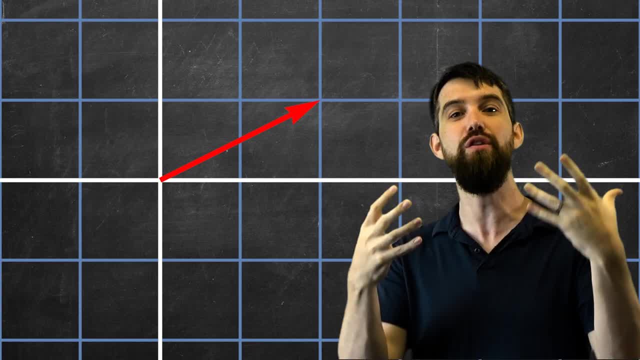 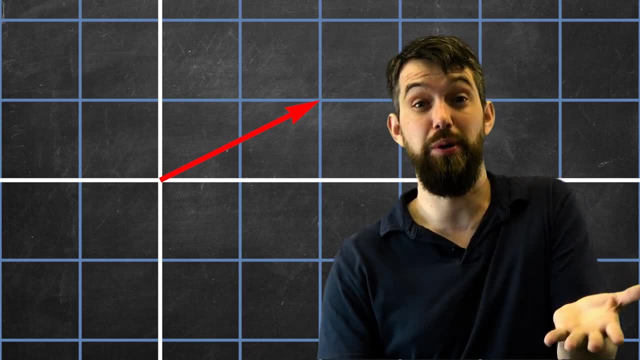 I may put the origin where I am and you may put the origin where you are, But either way, there's the same claim. It takes two steps to the right and one step up. All right, so I have these vectors, but what can I actually do with them? 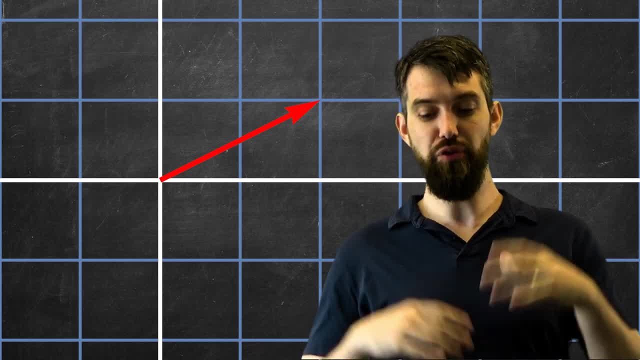 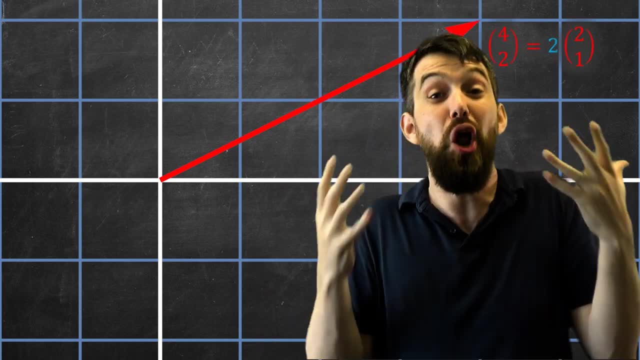 Well, one thing that I can do with them is I can stretch them. So, for example, if I take that same vector, the 2, 1, and I stretch it out by a multiple of 2,, I get this much larger vector, this vector 4, 2.. 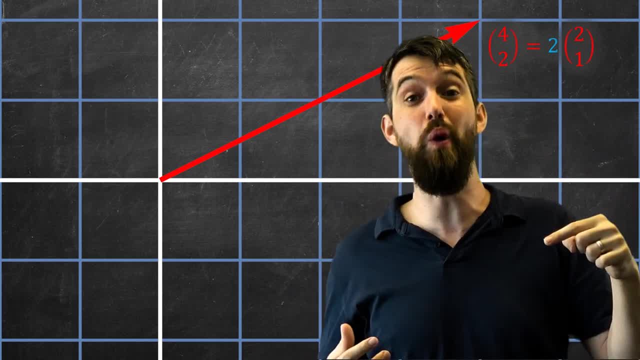 And basically what I've done here is that each of the components- the 2 and the 1, I've multiplied them by 2, and now I get to the point 4, 2.. This is a vector starting at the origin and going out. 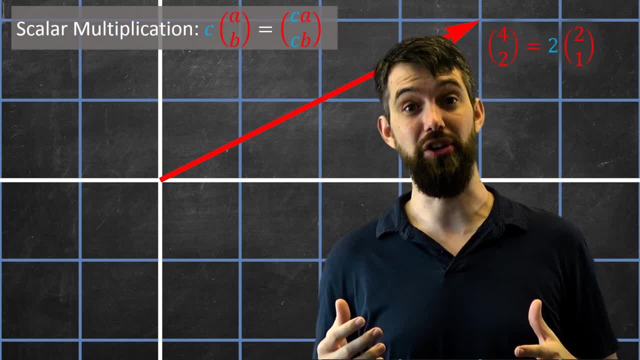 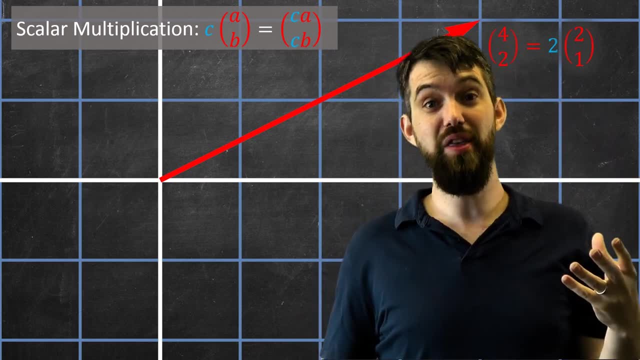 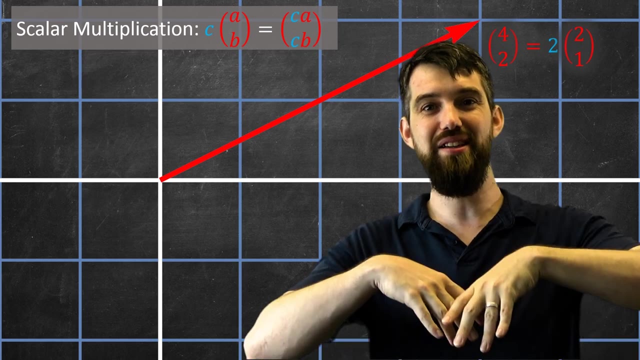 This is referred to as scalar multiplication and basically the idea is that if I multiply some vector by a scalar like number 2, then I multiply all the components of the vector by that scalar. I multiply them in this case by the number of 2, and the way I geometrically interpret. 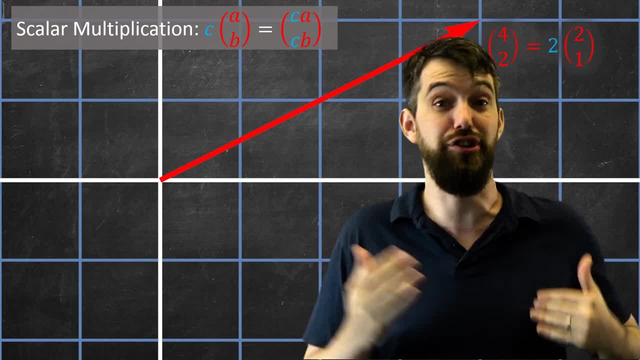 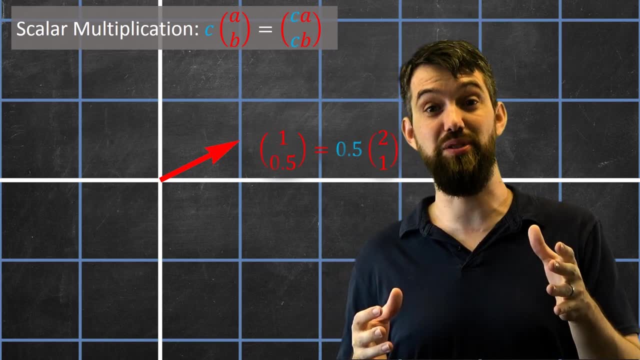 that is that it then takes the length of that vector doesn't change its direction, it's still pointed in the same place, but it makes it be twice as long. So, for instance, if c was equal to a half, I get then this much shorter vector. 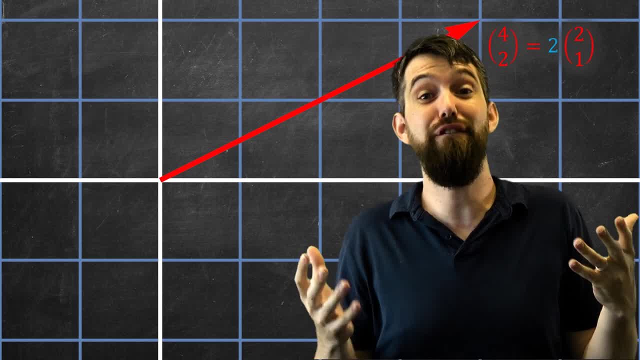 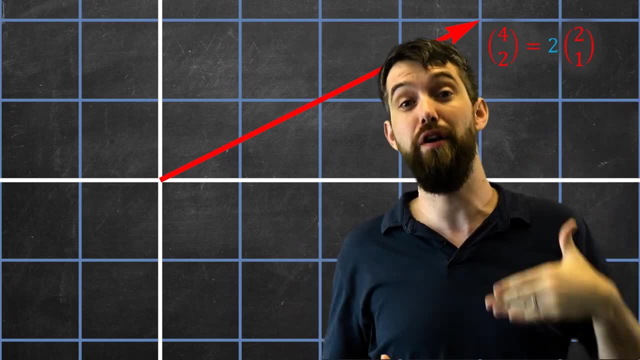 I get this much larger vector. this vector, And basically what I've done here is that each of the components- the 2 and the 1, I've multiplied them by 2, and now I get to the point 4, 2.. This is the vector starting at the origin and going out to 4, 2.. 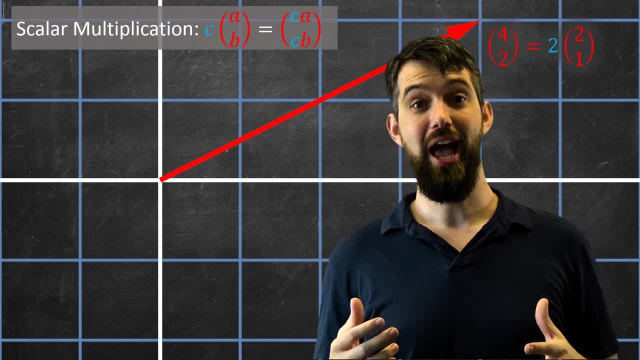 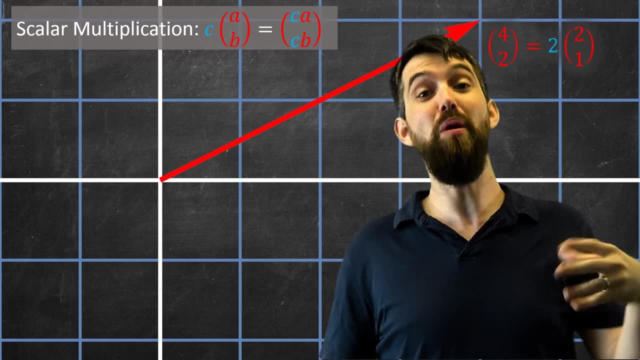 This is the vector starting at the origin and going out to 4, 2.. This is the vector starting at the origin and going out to 4, 2.. referred to as scalar multiplication, And basically the idea is that if I multiply some vector by a scalar like number 2, then I multiply all the 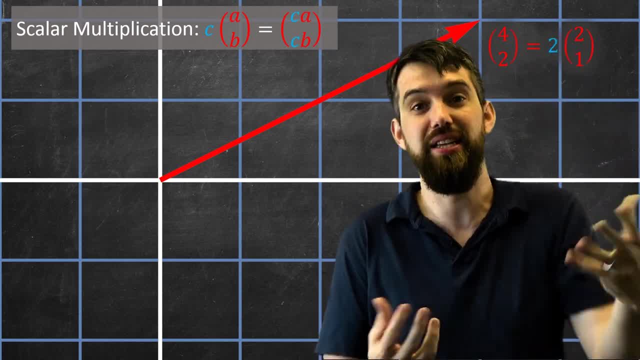 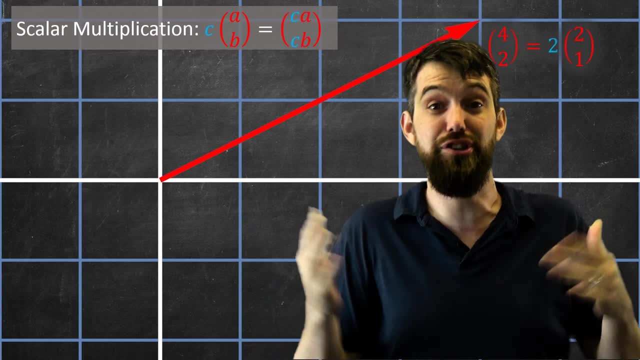 components of the vector by that scalar. I multiply them in this case by the number of 2.. And the way I geometrically interpret that is that it then takes the length of that vector doesn't change its direction, it's still pointed in the same. 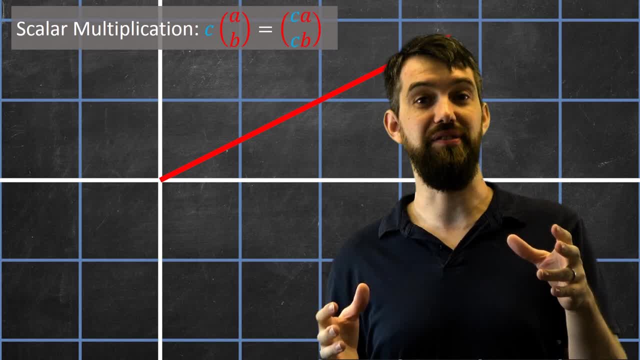 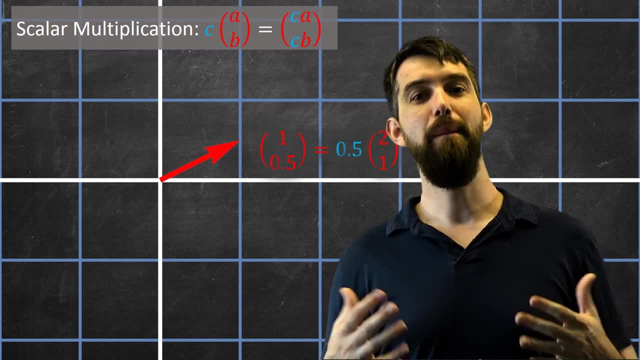 place, but it makes it be twice as long. So, for instance, if c was equal to a half, I get then this much shorter little vector, Even more interesting than that, if c is equal to minus 1, well, I still get the vector that's pointing the same. 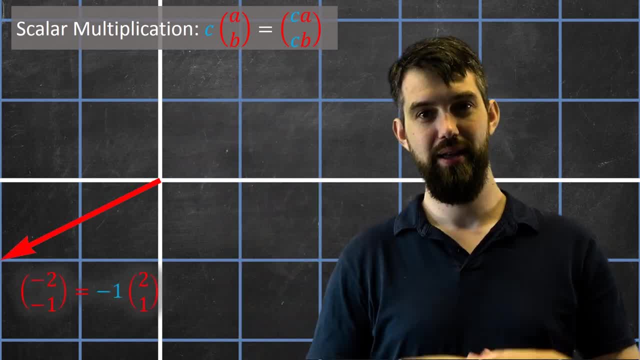 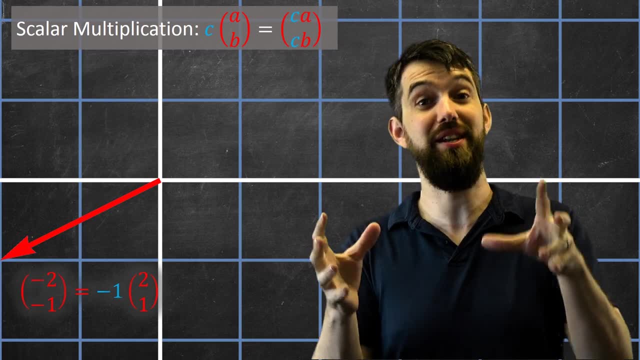 direction, or at least it's pointing to the exact opposite of it. And so when multiplying by a scalar minus 1, I get this vector minus 2, minus 1.. So that was one thing that I could do with the scalar multiplication. What's another? 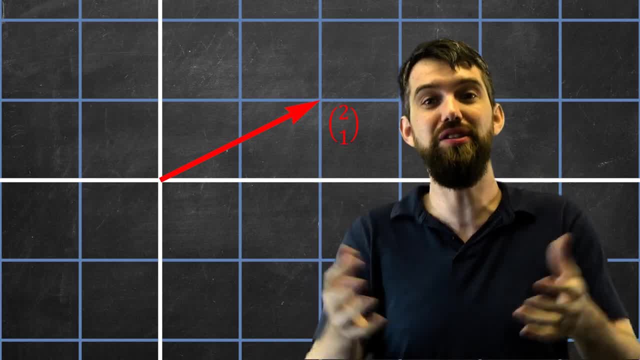 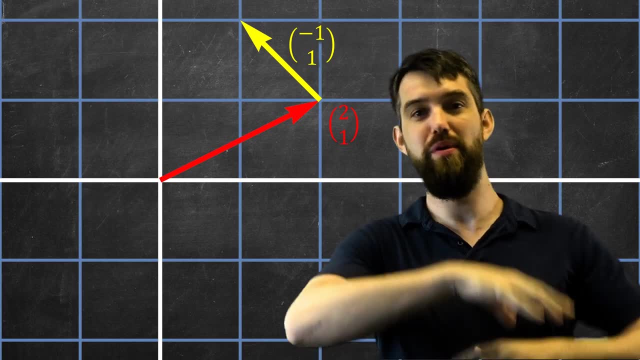 thing. Okay. so I want to see how I can combine different vectors. I've got this 2,1.. Let me add to this a second vector, the vector 1,1.. minus 1, 1.. Now, remember, vectors can move wherever I want. so I can take that minus 1, 1 if I prefer to think of it as 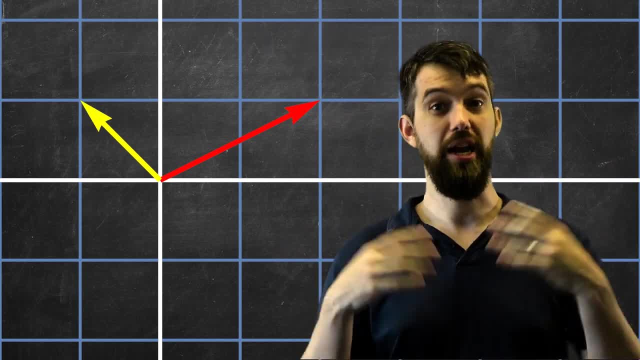 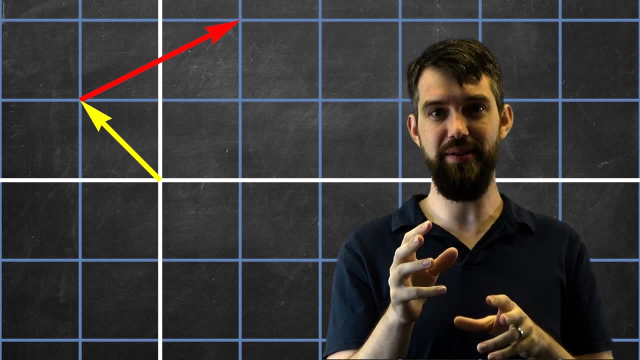 starting at the origin and going up from there. That's perfectly fine, And likewise I can move around the 2, 1 vector. I could shift that one up. Now, what I want you to pay attention to is that, right now, 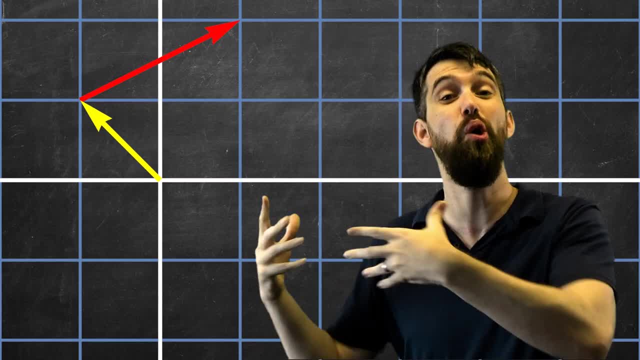 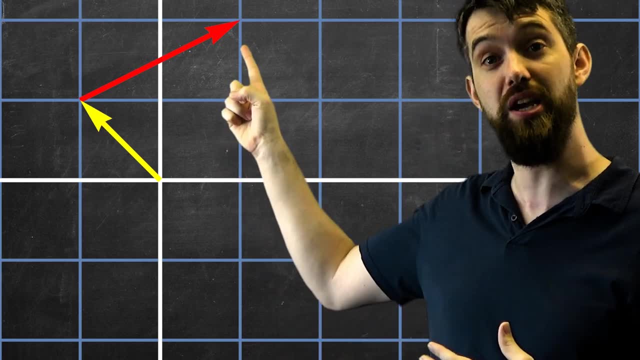 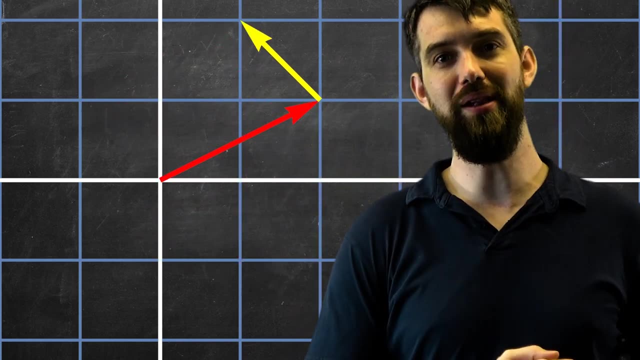 I've aligned these vectors in a sort of tip-to-tail way, that the end of the yellow vector is the start of the red vector and it goes up to this particular point right here, this point 1, 2.. Now, if I rearrange where these vectors are going to be, well, 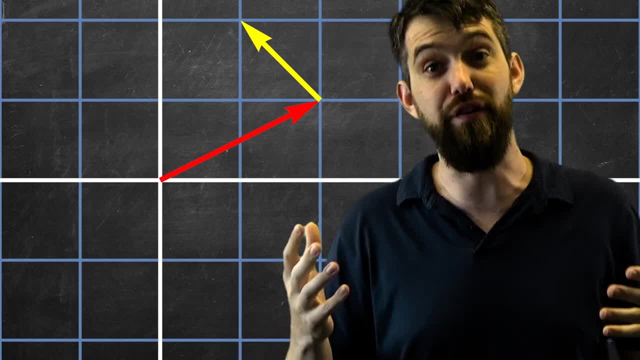 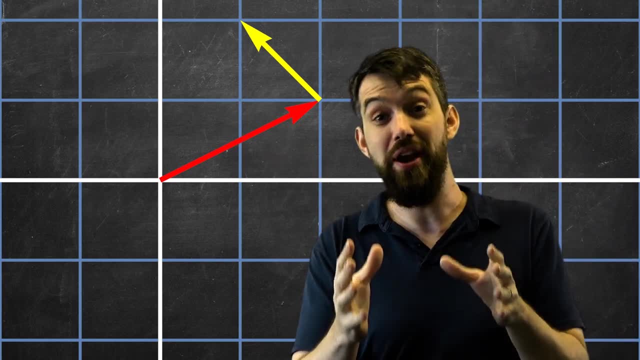 I still add them up in a tip-to-tail way, but I go the red one first and then the yellow one next, but notice how it still goes to that same point. It still ends at that 1, 2.. This is the notion of vector addition. 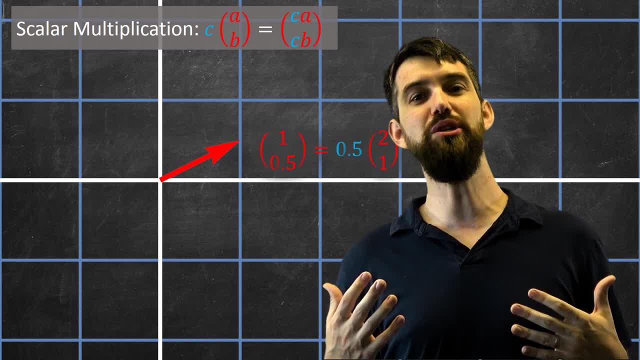 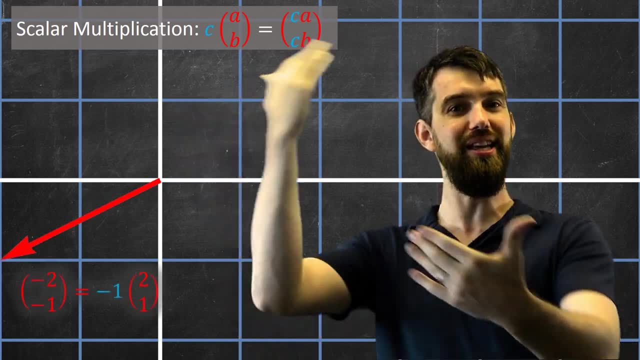 Even more interesting than that, if c is equal to minus 1,, well, I still get the vector that's pointing in the same direction, or at least it's pointing in the exact opposite of it. And so, when multiplying by the scalar minus 1, I get this vector minus 2, minus 1.. 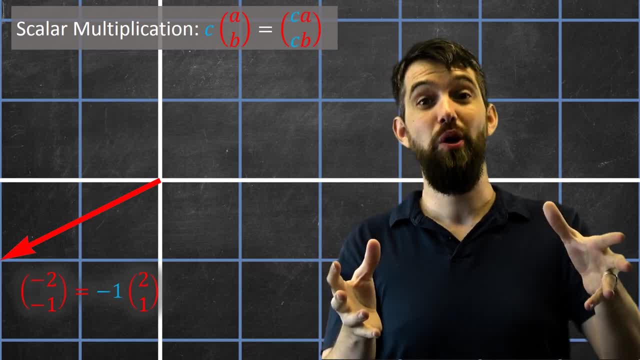 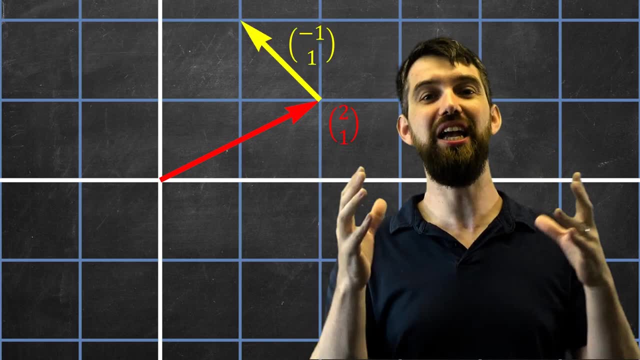 So that was one thing that I could do with this scalar multiplication. What's another thing? Okay, so I want to see how I can combine different vectors. I've got this: 2, 1, and let me add to this a second vector, the vector minus 1, 1.. 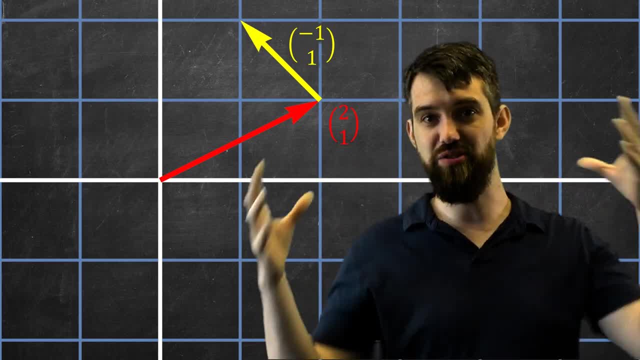 Okay, so I've got this 2,, 1, and let me add to this a second vector, the vector minus 1, 1.. Now, remember, vectors can move wherever I want, so I can take that minus 1,, 1, and. 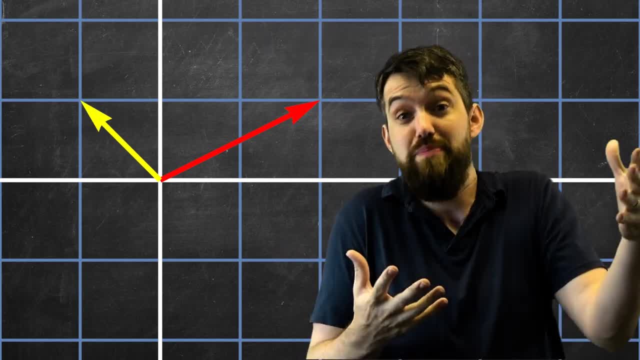 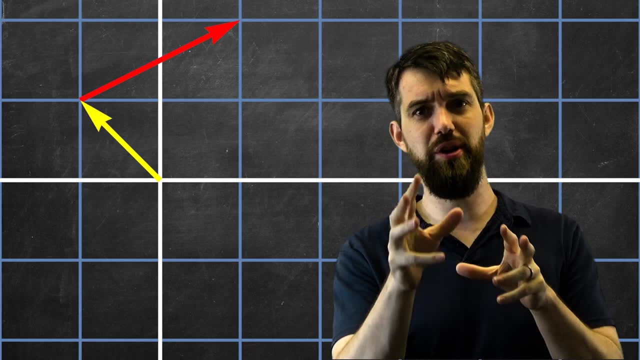 if I prefer to think of it as starting at the origin and going up from there, that's perfectly fine, And likewise I can move around the 2, 1 vector. I could shift that one up. Now, what I want you to pay attention to is that right now I've aligned these vectors. 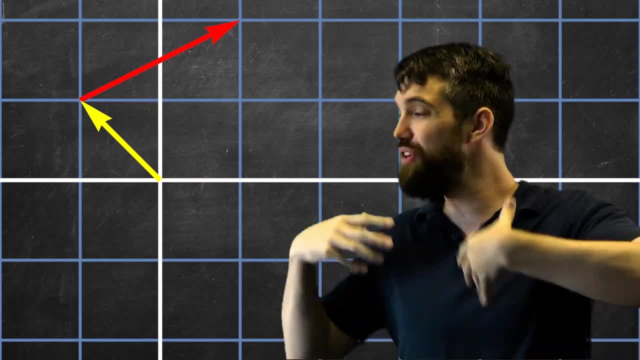 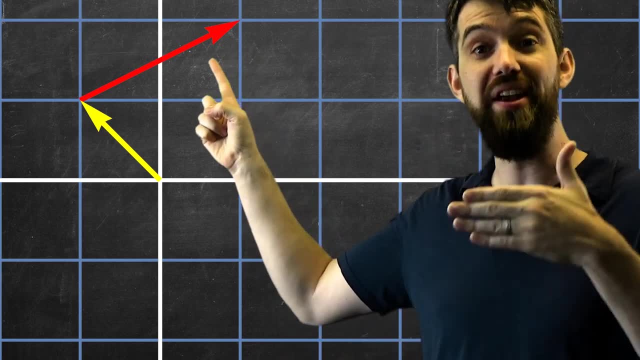 in a sort of tip-to-tail way, that the end of the yellow vector is the start of the red vector, and it goes up to this particular point right here, this point 1, 1.. Now, if I rearrange where these vectors are going to be, well, I still add them up in. 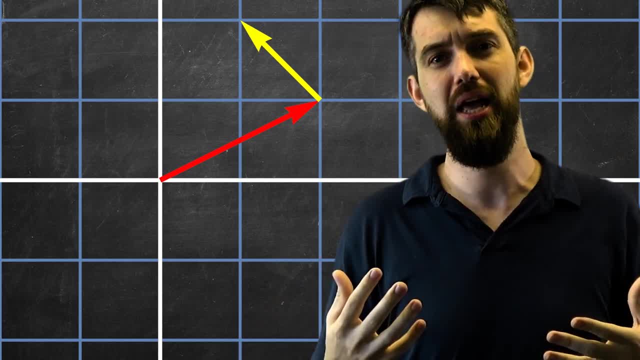 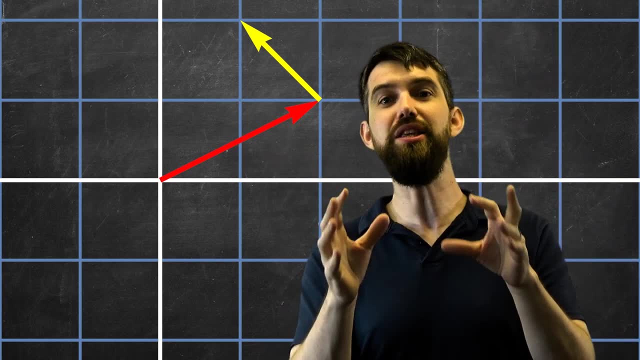 a tip-to-tail way, but I go the red one first and then the yellow one next, but notice how it still goes to that same point. It still ends at that 1, 2.. This is the notion of vector addition. 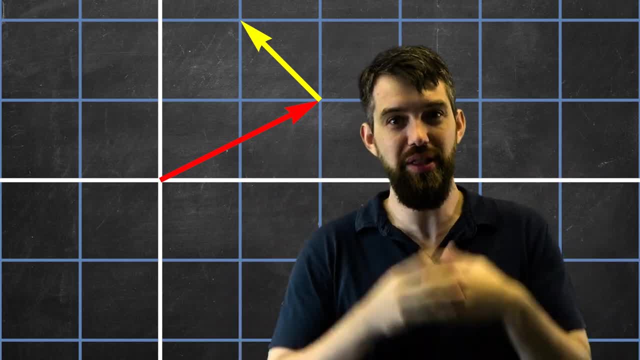 It tells me how can I- so-called- add two different vectors? and the answer is that you line them up in this tip-to-tail way And then I'm going to add these vectors. Okay, so I'm going to add these vectors. 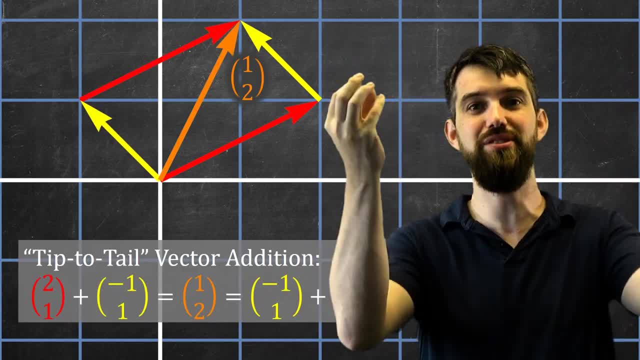 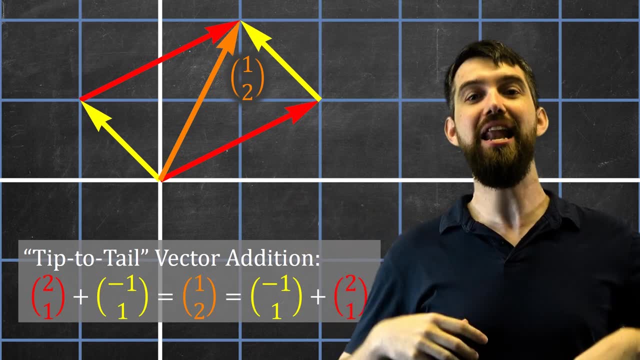 Algebraically, what that corresponds to is that when I'm adding these two vectors, I add them component by component. So I add up the first two, the 2 and the minus 1, and I get a 1, and then I add up the second. 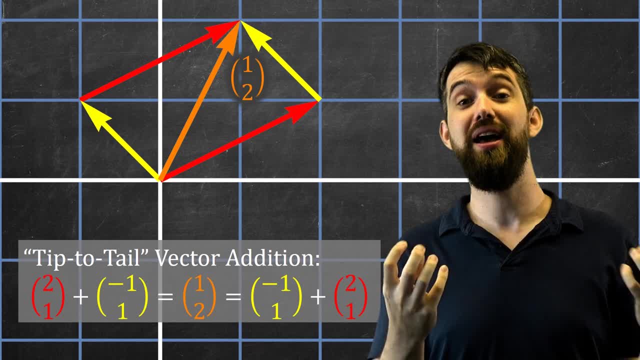 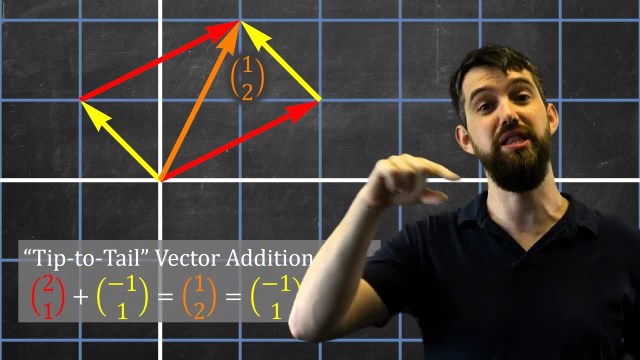 components, the bottom components. I'm going to take a 1 and a 1, and I'm going to get 2.. And then notice how geometrically it didn't matter whether we went the yellow first and the red second, or the red first and the yellow second, that it didn't matter whether we commuted. 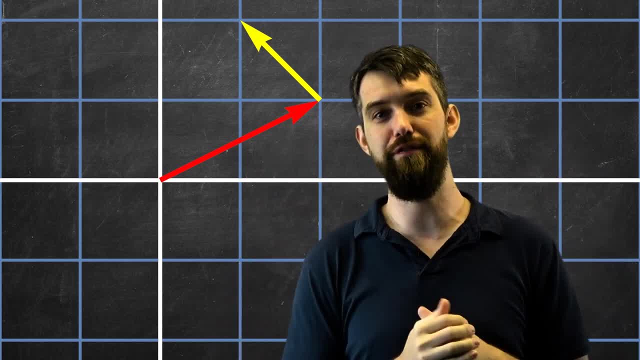 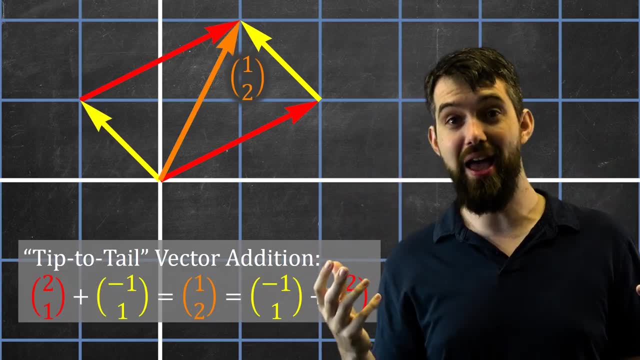 It tells me how can I- so-called- add two different vectors, and the answer is that you line up them up in this tip-to-tail way And then, algebraically, what that corresponds to is that when I'm adding these two vectors, I add them component by component. 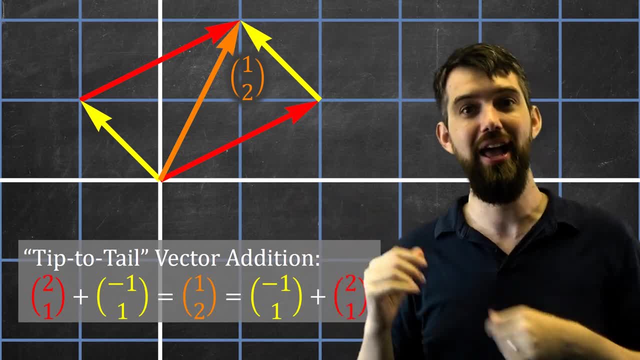 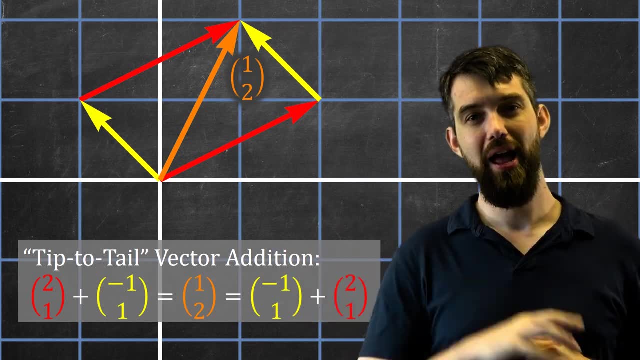 So I add up the first two, the 2 and the minus 1, and I get a 1.. And then I add up the second components, the bottom components. I'm going to take a 1 and a 1, and I'm going to get 2.. And then notice how. 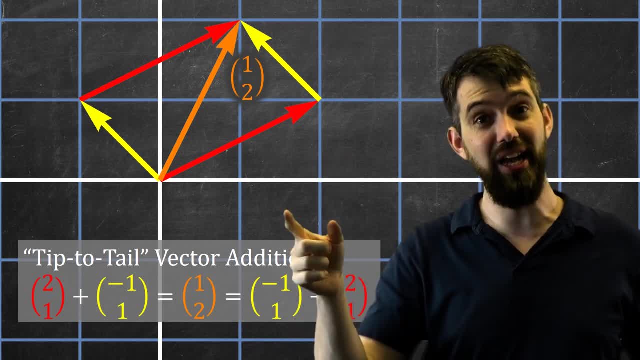 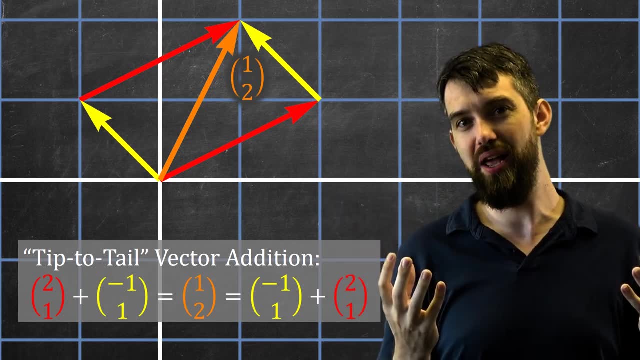 geometrically, it didn't matter whether we went the yellow first and then the red second, or the red first and the yellow second, that it didn't matter whether we commuted the order of which our tip-to-tail addition was going on. We see the same thing. 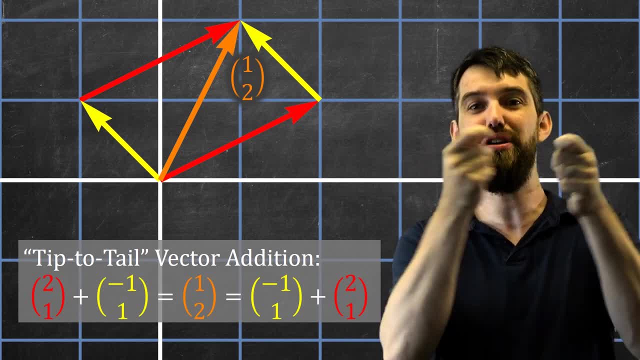 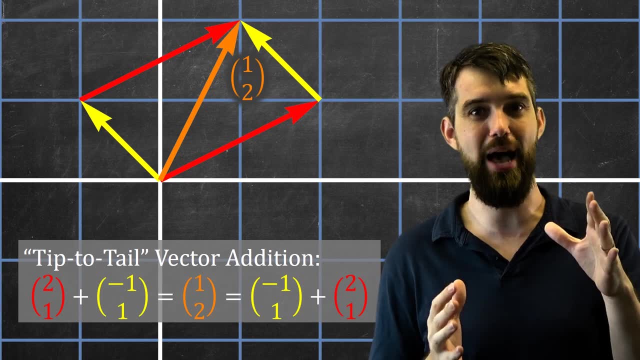 algebraically It doesn't appear to make a difference here because addition of numbers- I can switch that order around. So whichever order it gets to this same vector, It's always really nice when this happens, when we've got this geometric picture of what addition means, this tip-to-tail alignment of these vectors. 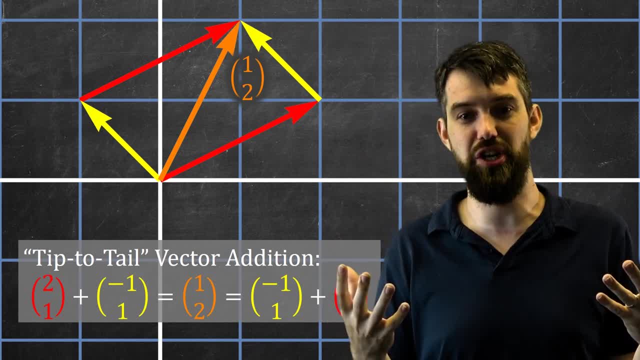 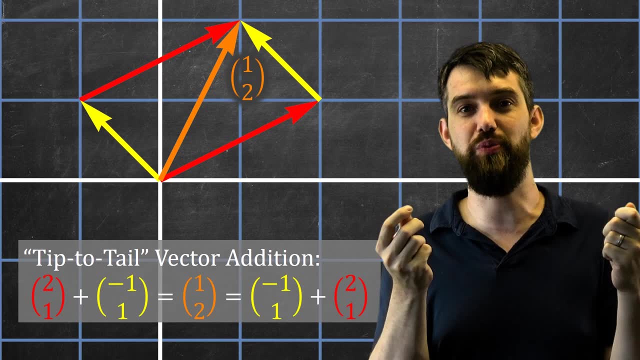 And then we have this algebraic definition of vector addition, where I combine them in this way, adding them up component-wise, And then the property that we can commute, the order of adding our vectors. we see that both algebraically and geometrically. 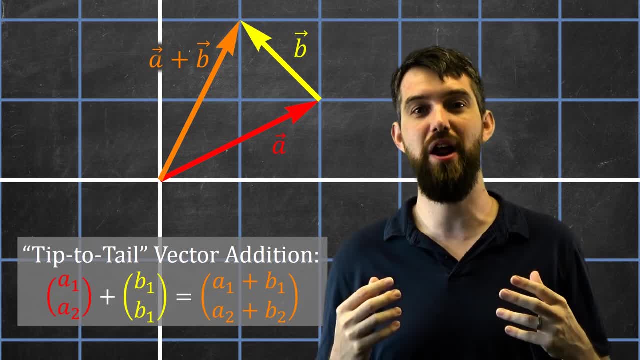 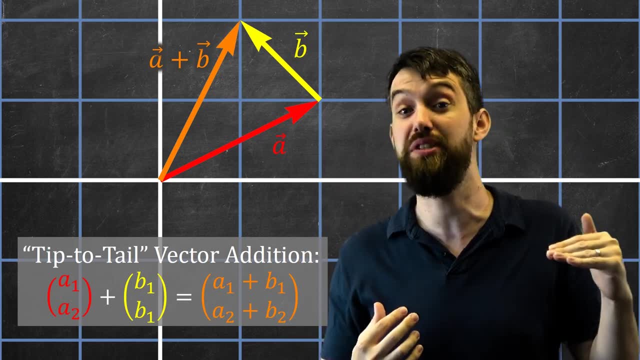 More generally, this is how I define my tip-to-tail addition where I've got an a vector and a b vector. Geometrically they add up tip-to-tail and algebraically you take the a1, a2, the components of the a vector and the b1, b2,. 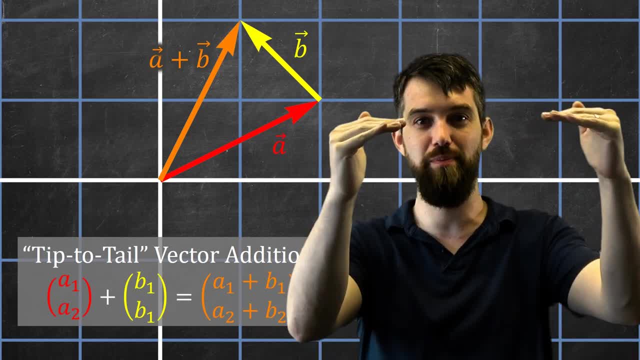 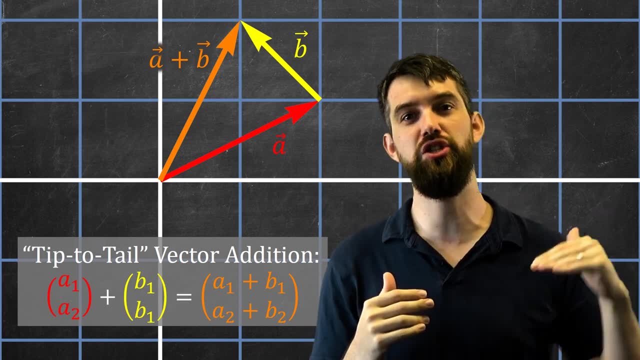 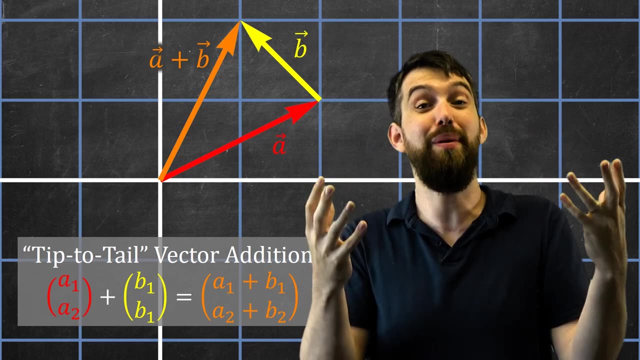 the components of the b vector and you add them component-wise: a1 plus b1, a2 plus b2.. So these two different operations that we have, scalar multiplication that stretches a vector by some scalar and vector additions where I add them up tip-to-tail. these are the two basic ways I'm allowed to manipulate and change. 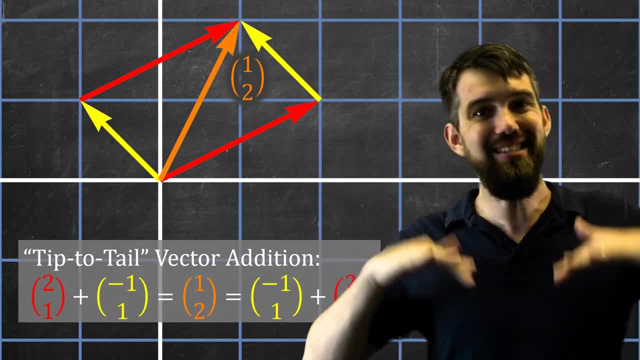 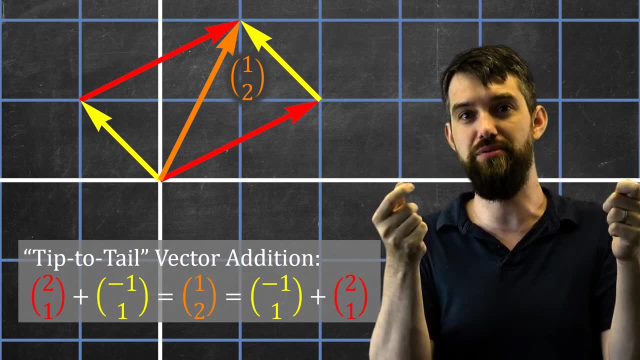 the order of which our tip-to-tail addition was going on. We see the same thing algebraically. it doesn't appear to make a difference here because addition of numbers. I can switch that order around, So whichever order it gets to this same vector. 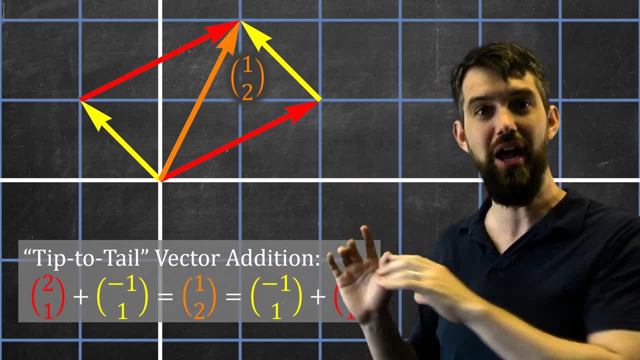 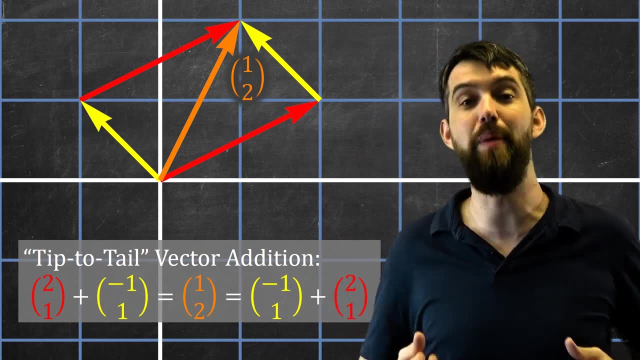 It's always really nice when this happens, when we've got this geometric picture of what addition means, this tip-to-tail alignment of these vectors. And then we have this algebraic definition of vector addition, where I combine them in this way, adding them up component-wise. 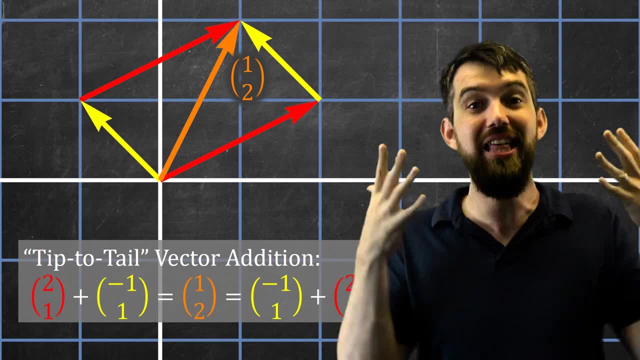 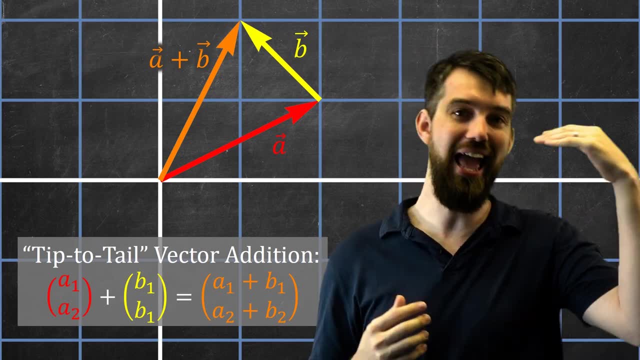 And then the property that we can commute, the order of adding our vectors. we see that both algebraically and geometrically. More generally, this is how I define my tip-to-tail addition where I've got an a vector and a b vector. geometrically they add up tip-to-tail and algebraically you take the a1, a2, the. 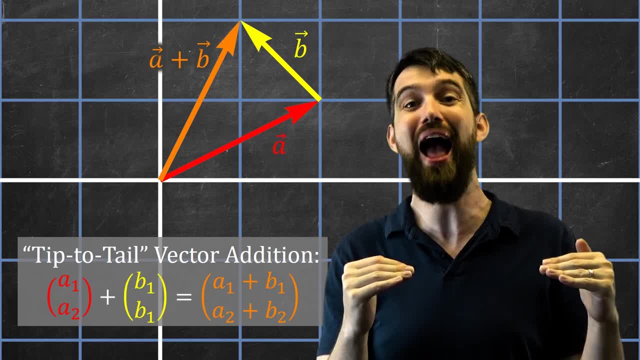 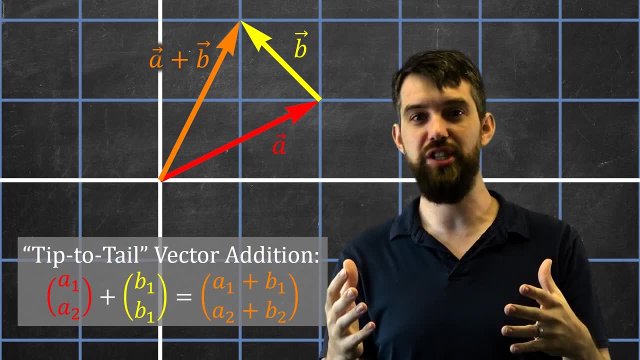 components of the a vector and the b1, b2, the components of the b vector and you add them component-wise: a1 plus b1, a2 plus b2.. So these two different operations that we have, scalar multiplication that stretches. 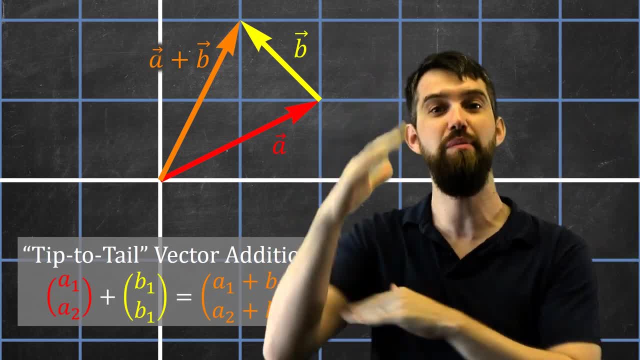 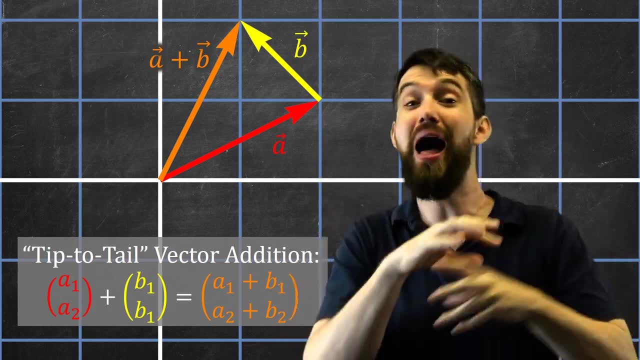 a vector by some scalar and vector additions, where I add them up tip-to-tail. these are the two basics. These are the basic ways I'm allowed to manipulate and change vectors, the way I can combine different vectors. In the next video we're going to go and take it one next step further and we're going: 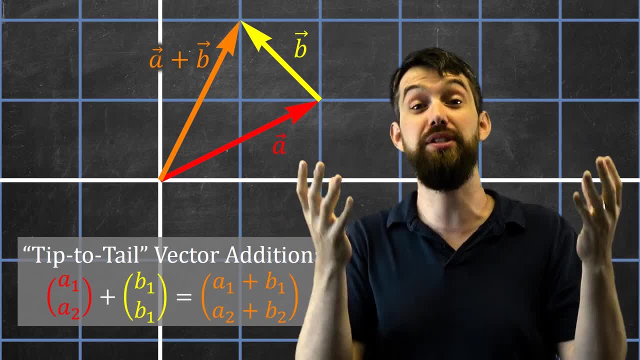 to look at all the possible ways that I can combine vectors and trying to study that.